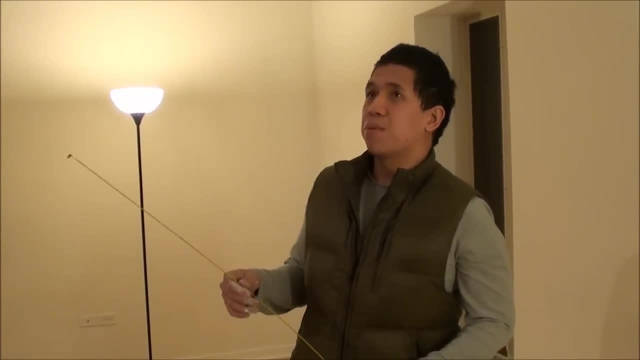 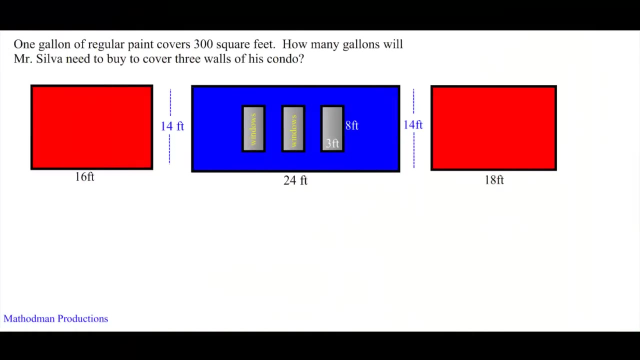 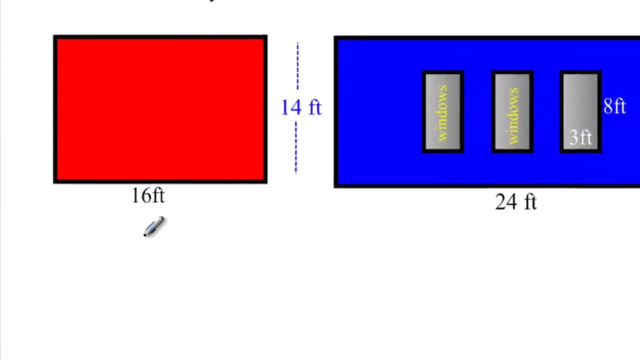 I just finished measuring all the parameters in my wall. Let's now take that result and relate it to surface area. One gallon of regular paint covers 300 square feet. How many gallons will I need to buy in order to cover three walls in my condo? 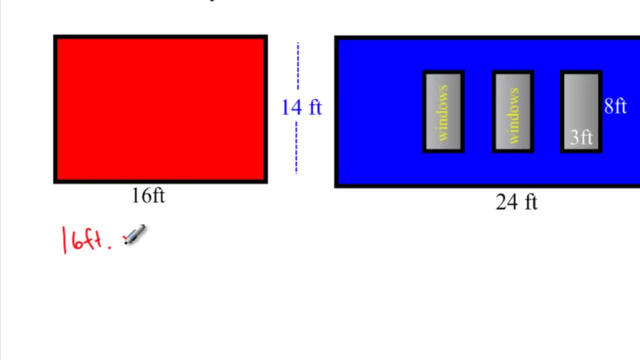 In order to do this, first I need to find the surface area of all three of my walls. Do the first red wall right here? To find it, all you have to do is multiply 16 times. Multiply 16 times 14 to find the surface area for that first wall. 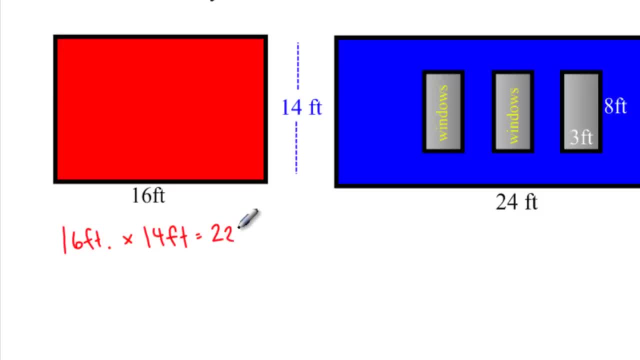 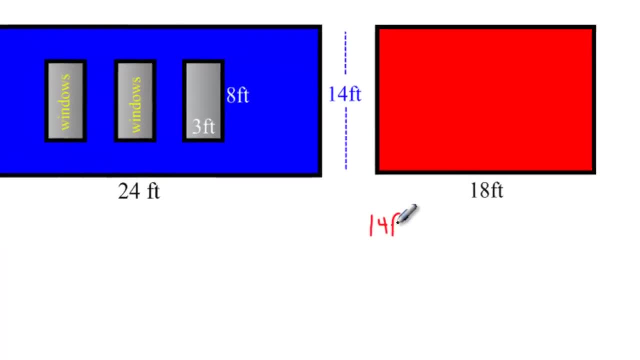 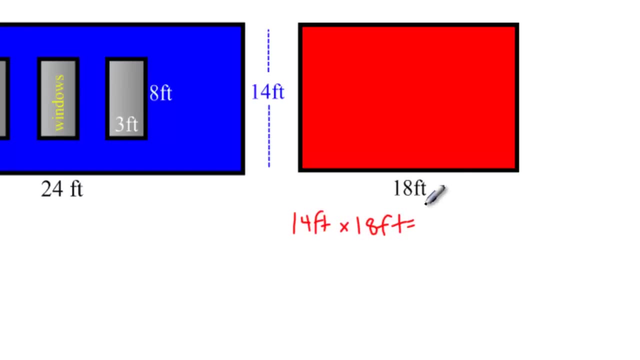 16 times 14 is just 224 square feet. We'll skip the blue wall for now To find the surface area of the red wall. we're still using the same formula for the area of a rectangle: 14 times 18 is going to be 252 square feet. 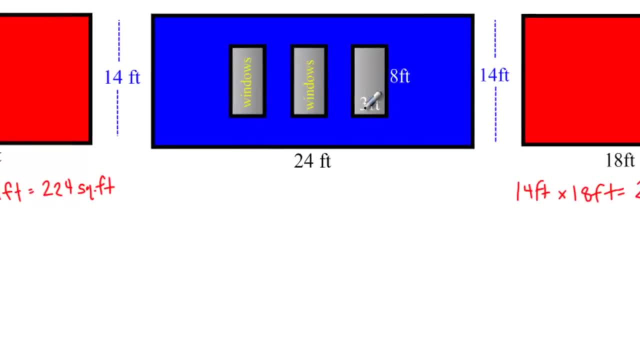 Now this wall in blue has three windows in it. Obviously, we're not going to paint these windows, So first find the area of the big piece, the big blue wall, by using the formula of a rectangle: 24 times 14 feet is going to be 336 square feet. 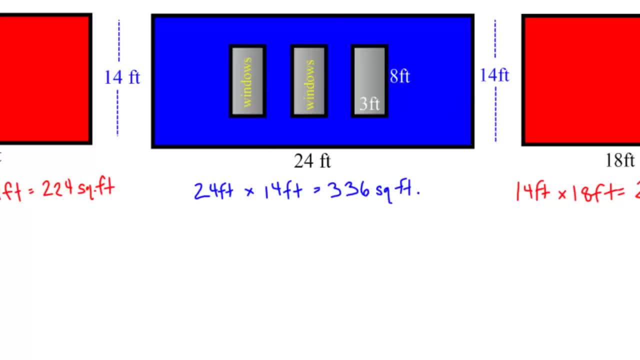 We're not going to paint the windows, but we still need to find the area for all three of them. They're all identical, so all I have to do is find the area of one window and then multiply it by 3.. Each window is a rectangle, so to find the area of one window, all I have to do is multiply 8 by 3.. 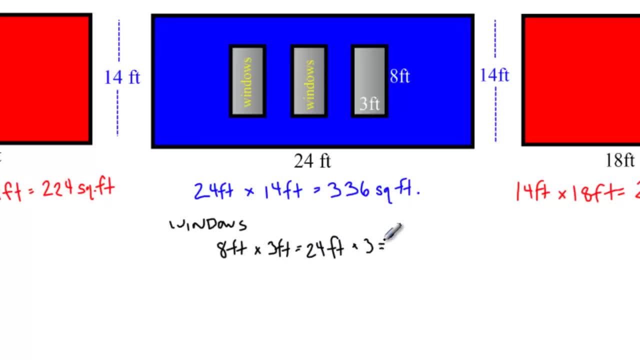 And I get 24 square feet. But then I have to multiply it by 3 again because there's three windows. So the total surface area for the three windows is 72 square feet. To find my total surface area it's pretty easy. 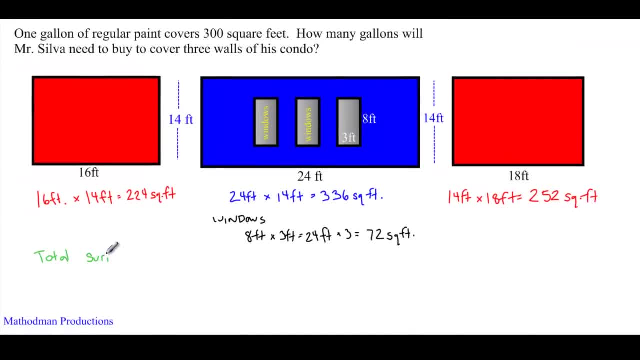 I just have to add up all the areas, the walls that I have to paint: The red wall, the blue wall and the other red wall. So I'll just add up all the pieces that I did: 224 plus 336 for the blue wall and the other wall is 252.. 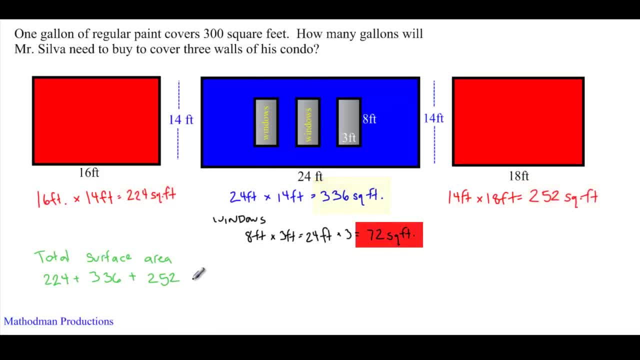 But the thing is I'm not going to add 72 because I'm not painting the windows, So I have to subtract. I have to subtract it from my total surface area. Make your calculations and you should get 740 square feet, Meaning I have to paint 740 square feet of my wall. 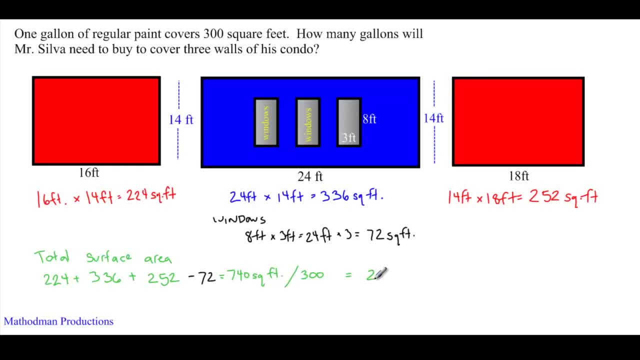 The last step is just to divide it by 300 square feet, because that's how much one gallon covers, And I figure out how many gallons of paint I have to buy: 2.46, repeating, I don't know that amount of paint exactly. 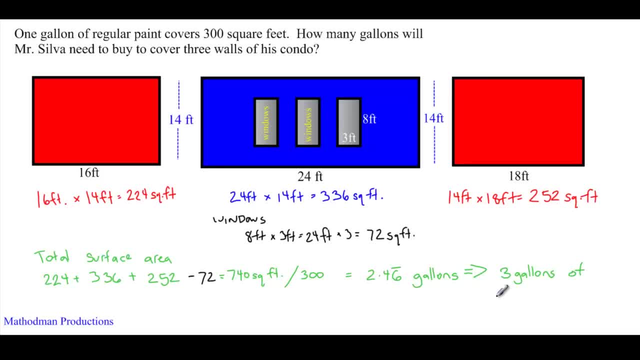 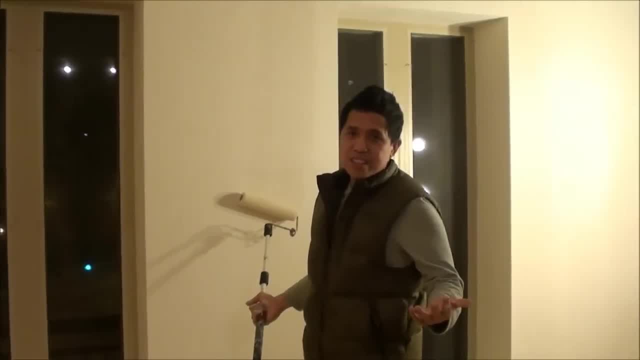 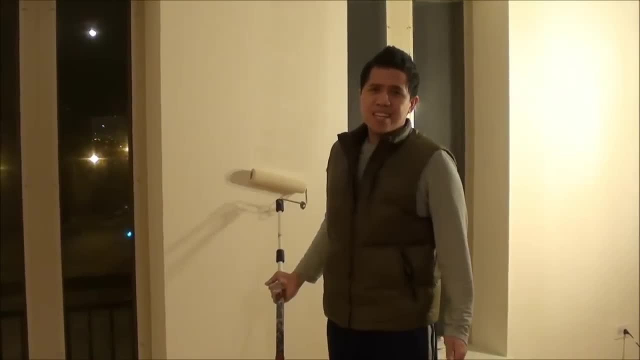 So I have to round it up to 3 gallons in order to paint all three walls of my condo. By using surface area, you can clearly estimate how much paint you'll need for a project such as painting your house. Now use your knowledge about surface area and try a problem on your own. 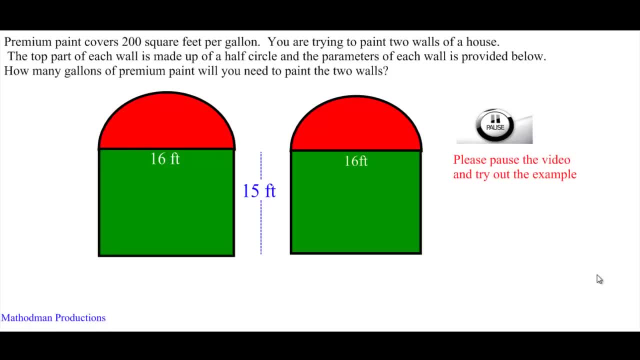 3.45. repeating. Premium paint covers 200 square feet per gallon. You are trying to paint two walls of a house. The top part of each wall is made up of a half circle And the parameters of each of the wall is provided below. 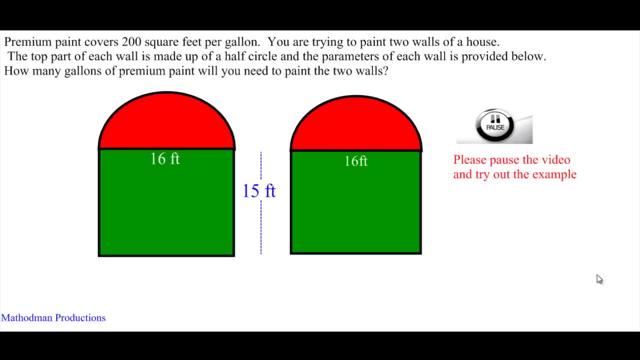 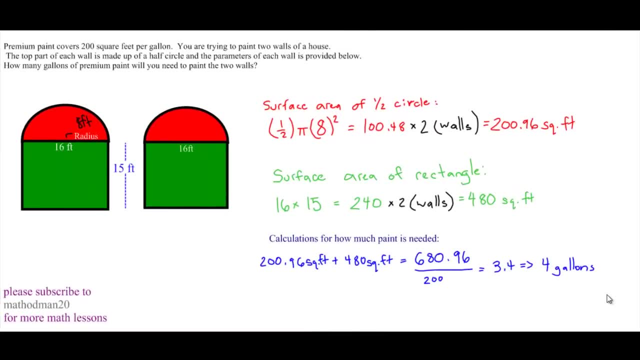 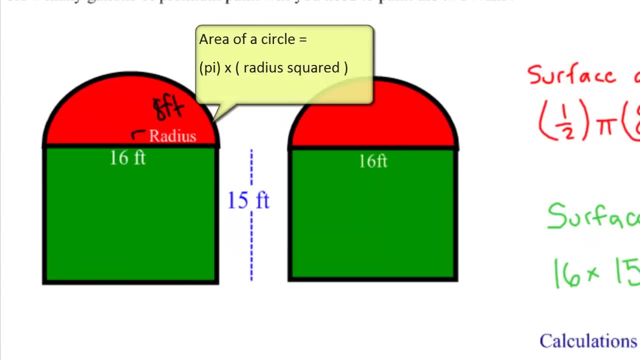 Please pause the video and try out the example. When you have finished, the answer will be explained right to you. In order to do this problem correctly, you need to know the area of a circle. I started by finding the surface area of my half circles. 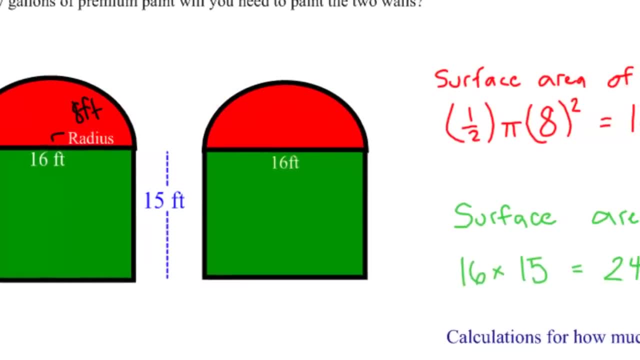 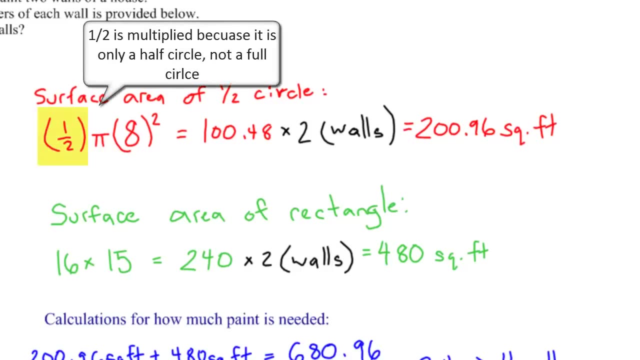 And since my diameter of 16 feet is given to me, I know that my radius is 8. So I did pi times 8, squared times a half, That equals to 100.48 square feet, And since there's two of them, I multiplied it by 2.. 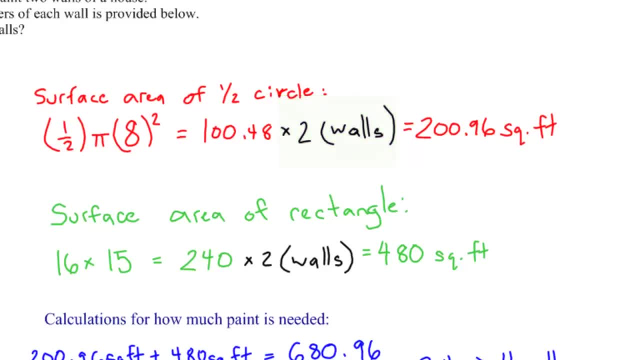 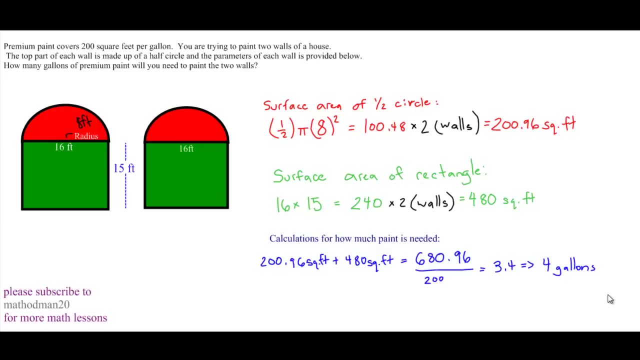 And I got 200.96 square feet for the red parts of my wall. The green parts is easy. Just find the area of a rectangle. That's just 16 times 15. Which equals to 240.. And since there's two of them, I multiplied it by 2..